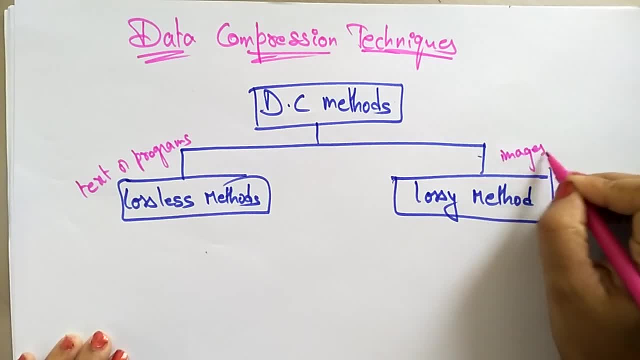 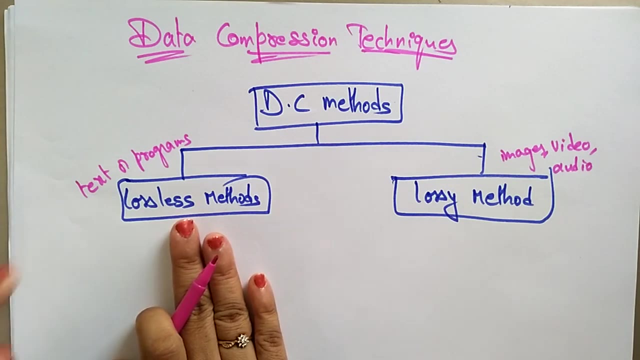 It is for Images, Videos And audio, We can go for the lossy method. So if you are doing the data compressions on the images, videos and audios, you can go for the lossy methods. And if you are using the data compressions on the text, if you want to compress the text, compressing means you want to reduce the size. Okay, so lossless method means the data will not be lost. 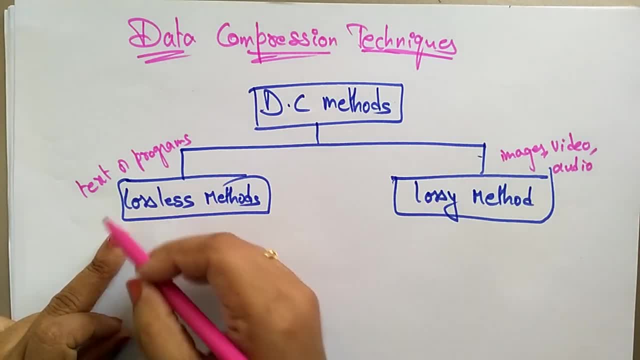 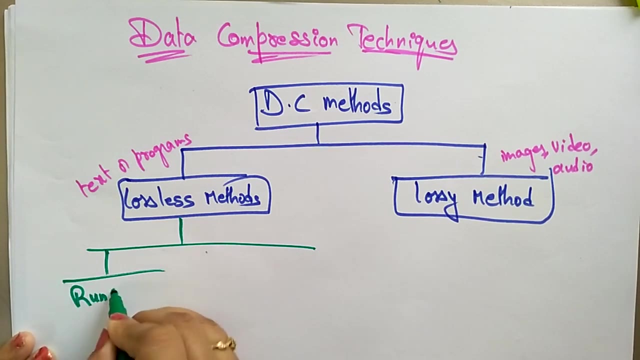 Whatever you are sending, that will be Received by the receiver. So the lossless methods will be performed on the text or programs. Okay, So again, this lossless the different types will be means the different techniques will be: run, length, run, length is a lossless method and Huffman. 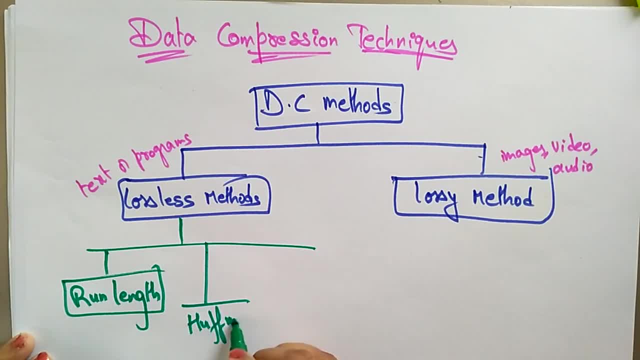 Huffman. Huffman method encoding is also a lossless method, and another technique here is the Lempel-Zeeb. Lempel-Zeeb is also a lossless method. This means one type of the compression. it's a lossless compression. data compression. Huffman is also one technique for the lossless. 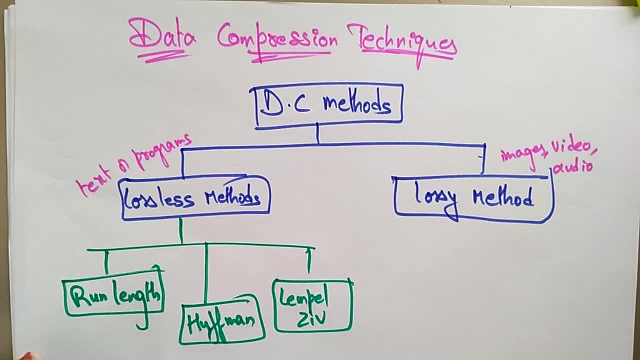 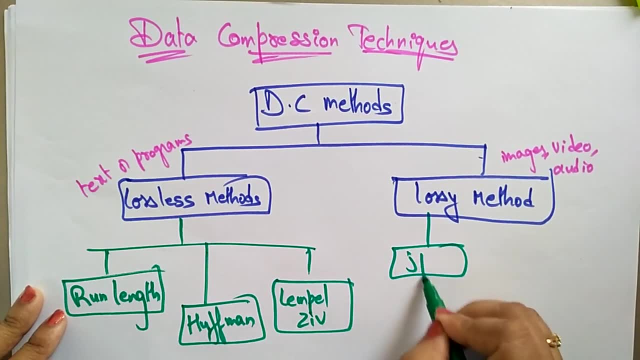 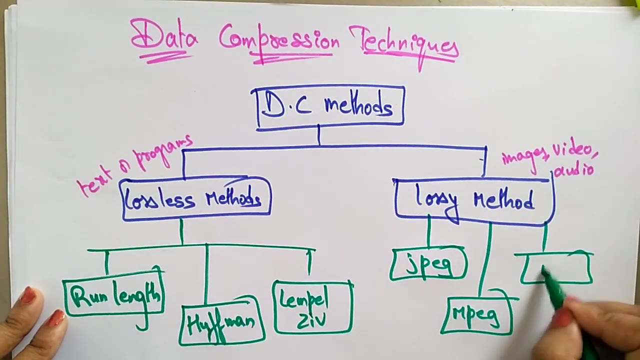 data compression and run length is also one type of the data compression. So that is a lossless and lossy methods are of JPEG, MPEG and MP3. So you already know about all these things. You had seen the what is jpeg files, mpeg files, mp3 files. You know only. 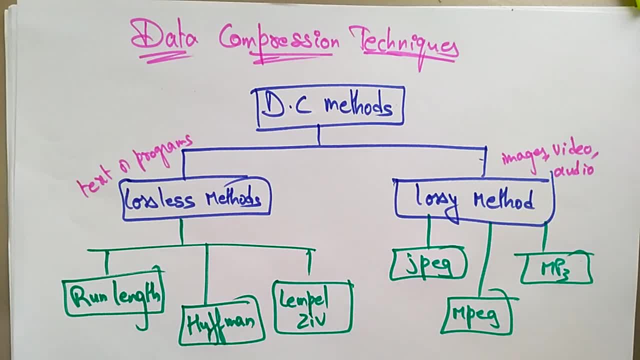 that thing. Okay. So here I am saying that these methods are lossy methods. Okay, By seeing this, you get a doubt. Okay, jpeg files contains a lossy information, or mp3 files make it's have a. 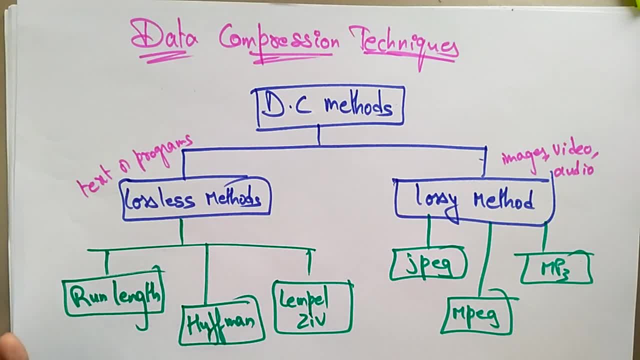 lossy information. Okay, It have a lossy information, but not that much. Only the unwanted data will be removed and compressed, So only the difference, but you can't able to identify what you are missing. also, It's just a minor thing. If you take the images, only the unwanted pixels. 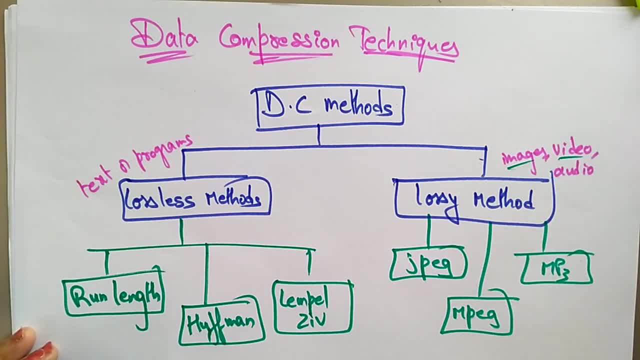 will be removed. If you take the video only the minute variation, your eyes will can't recognize what is a mistake there. Okay, Only that type of information will be removed. That is a lossy. That's why we call: these are all files. 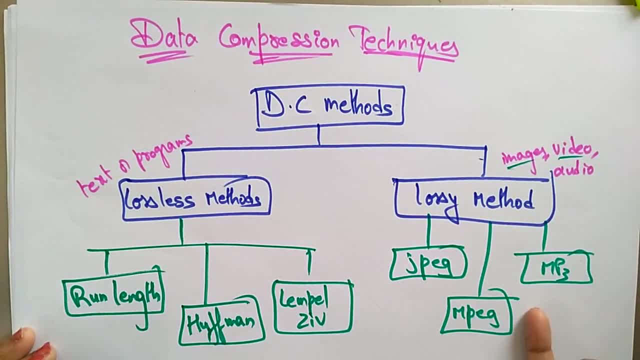 will have contains the lossy information, the lossy methods- Okay, So that lossy cannot be detected by the human eye- also, And lossless methods. the lossless methods is a run length: Huffman and Lempelgewe. Actually, these are lossless methods. means here the data can. 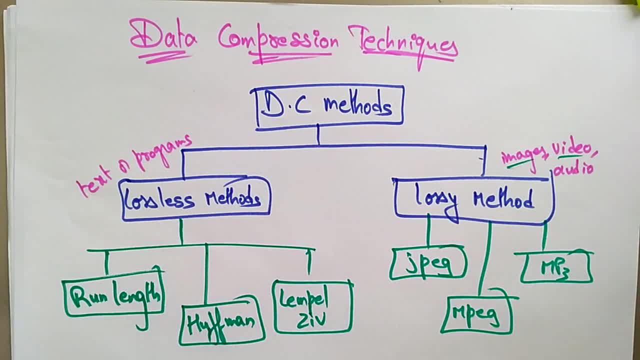 cannot be removed. Whatever the data that you want to be compressed and that data will received by the receiver after decompressed, the same data, whatever you send, means it having the redundant data. it contains redundant data Because it is a text or programs in the text you can't remove. 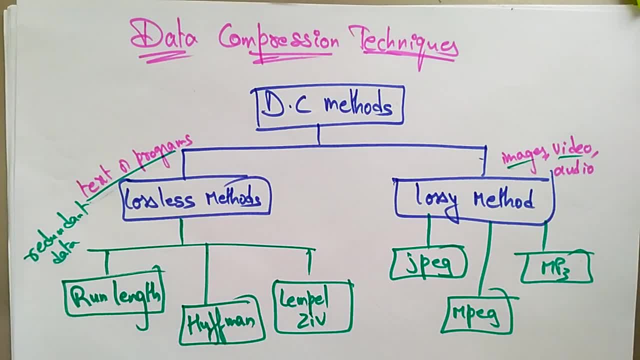 the letters, because you can't remove the redundant data. Maybe it will be helpful for the, the user. You can't remove that, So that's why we call the data compressions, while compressing the data, to send the data from sender to the receiver, for the sake of the storage and for the sake of the data. 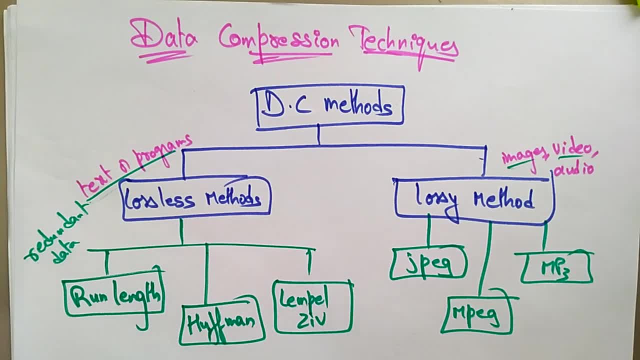 transmission. to make data transmission easy, we need to compress the files. Okay, So the files may be a text or a programs, or images, video, audio. So if you're taking the text or a programs, the text or programs, the data compression is a lossless methods. We use the lossless methods. 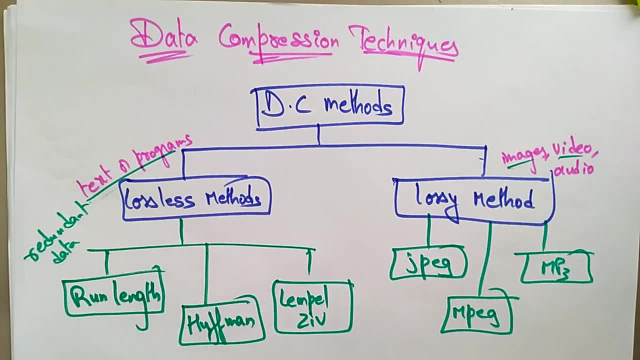 compress, Okay, So if you're taking the text or a programs, the text or programs, the data compression is a lossless methods. We use the lossless methods. We use the lossless methods Because whatever the sender wants to send, exactly that information will be received by the receiver. 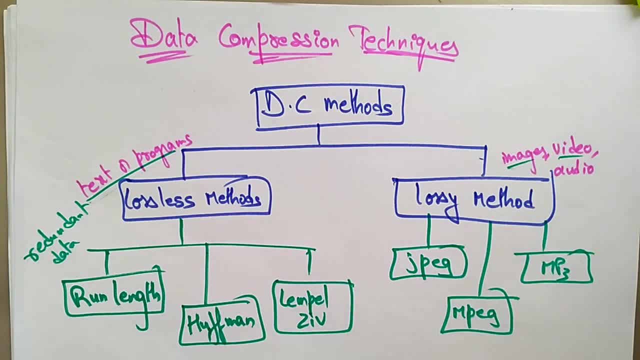 after delivering: Okay, Before compression and after compression, the same information will be there. Okay, Including the redundant data, So that we call it as a lossless. And there is a lossy means there may be a redundant data may be removed and that can't be recognized by the human eye. also. 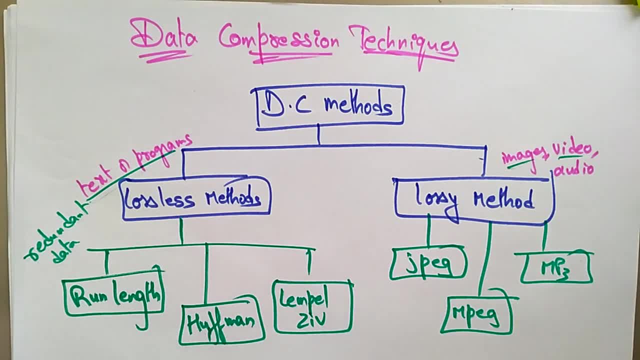 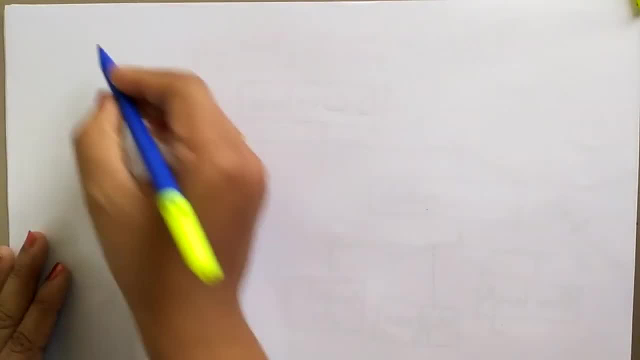 So that is a lossy methods. Okay, So the data compression methods are of two types: lossless and lossy. So let me explain you. before going to explain the techniques, let me give the clear idea: what is a lossless compression? 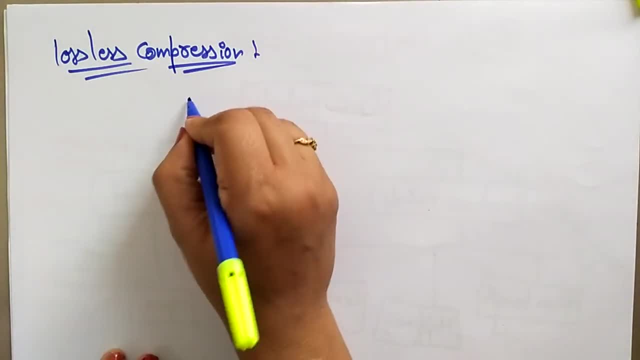 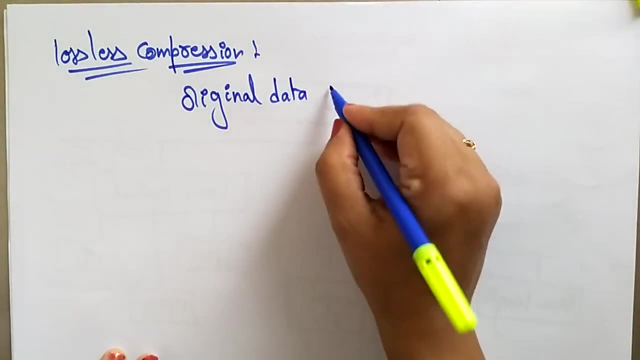 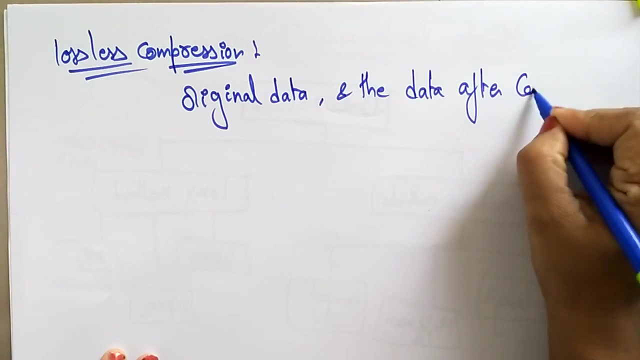 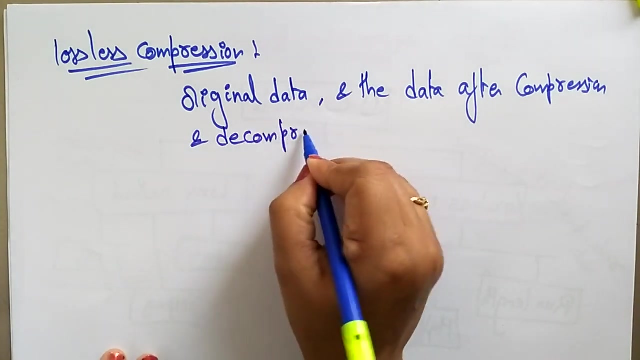 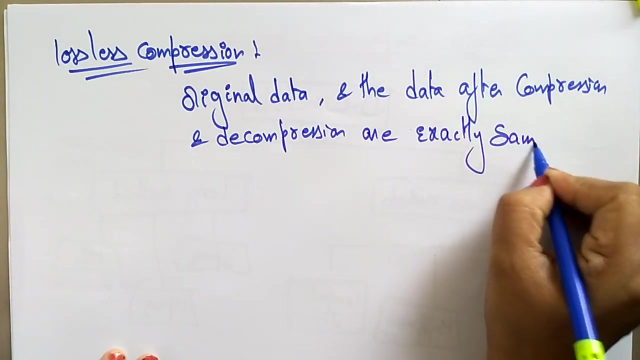 Lossless compression. A lossless compression is a original data. Okay, It's just a original data and the data after compression and decompression and the data after compression and decompression are exactly same, Exaclty same. okay, So, whatever the data that I am sending, 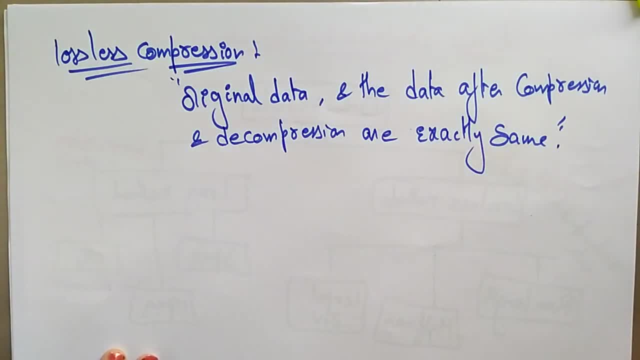 exactly the after decompression is also the same data will be there. Suppose I am sending Bhano Bhano In the receiver side also, you will get the Bhano Bhano, The same message. okay, i'm not removing the redundant data, i'm not removing the letters also, that is a lossless. 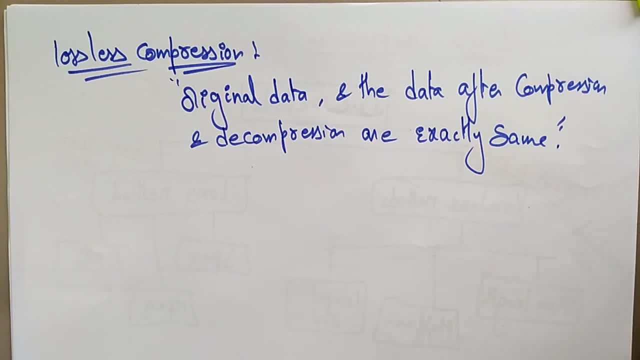 compression, the exactly same data, whatever you are compressed you want to send, that is, before compression and after decompression, is also the same data will be there here. redundant data is removed in compression and added during decompression, so you will get it out, okay, if you are not removing the redundant data, how the data will be compressed, how the data size will be. 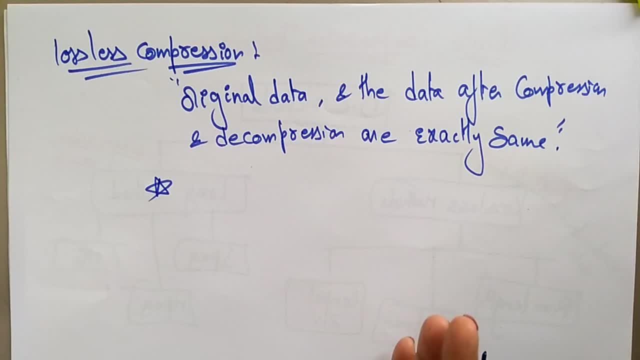 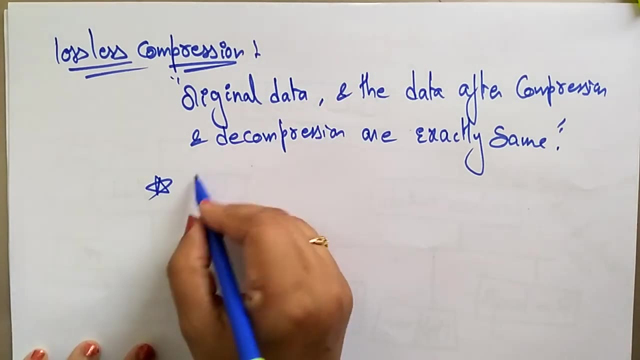 reduced when only you remove the redundant data, then only the data will be. uh size will be reduced, obviously, okay, so the if you remove the multiple data, then only the data file size will be reduced. so, without removing the redundant data, how it is possible? let me show you the redundant 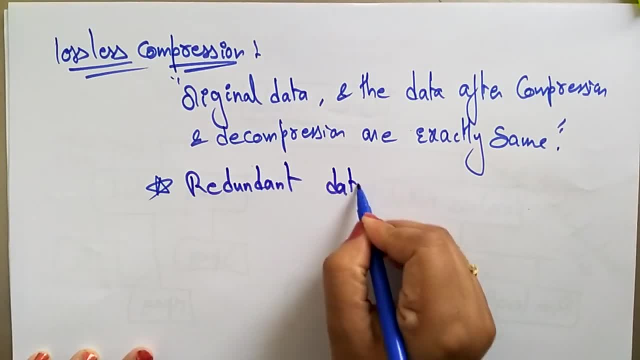 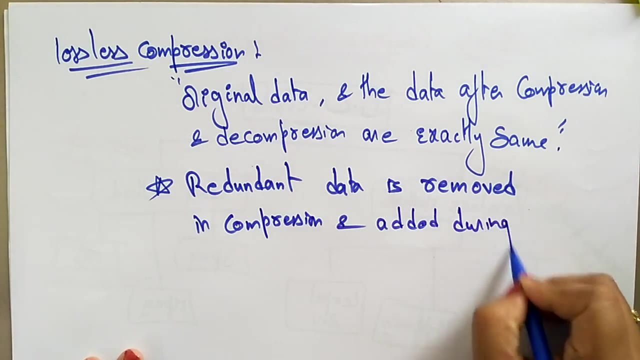 data is removed in compression. so while compression the redundant data is removed in compression. so while compression the redundant data is removed. the redundant data is removed in compression. so while compression the redundant data is removed and it will be added during decompression. did you get it means at the time of the uh compression? 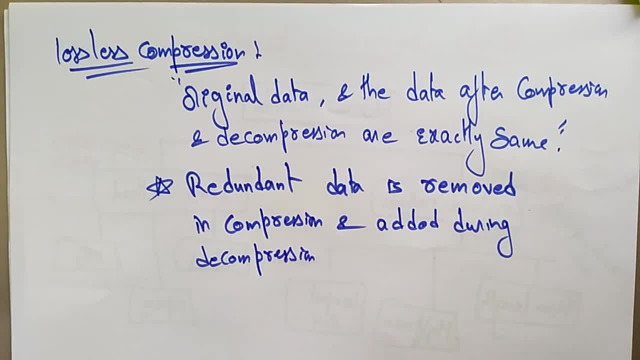 the remaining data will be removed means the in the place of that written data we are just including some numbers, suppose a, b, a, b, a, a, like this it is there. so here a, b, a, b is coming twice. so you are just writing two a b. so here instead of four letters, we are just writing three letters. 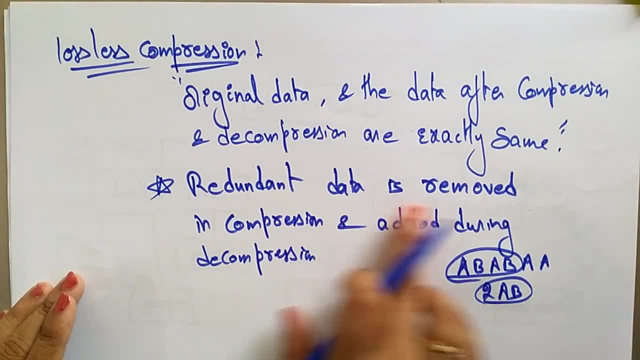 okay, so that will be the technique here. the redundant data is removed in compression and added after decompression. so during decompression again, in place of two a b, it's uh right, a, b, a b after decompression. so that is the technique of the lossless. so here we are. 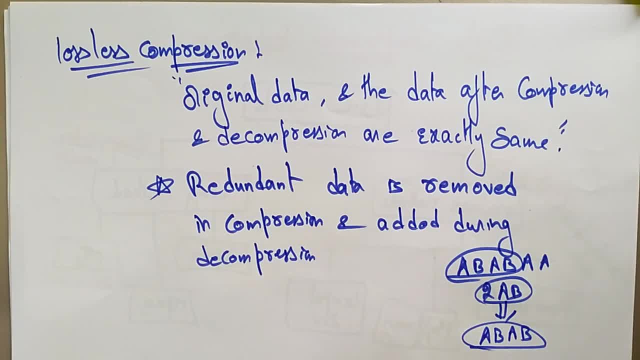 removing the redundant data while compressing. so if you didn't remove the redundant data while compressing, what happens? the file size will not be reduced, but our aim of the data compression is we need to reduce the size of the file. okay, so the lossless methods are used. 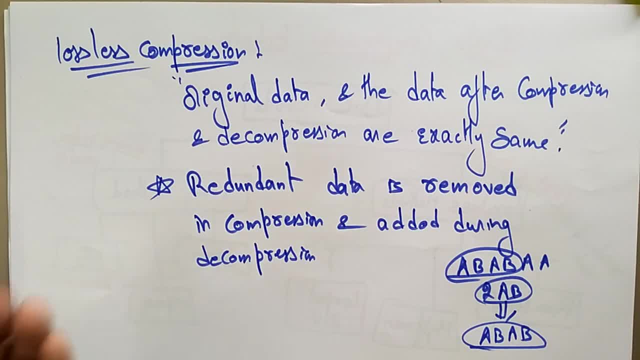 when we can't afford to loss any data. so in case of the legals and the medical documents and the computer programs, they we can't, uh uh, lose the data. so in that cases we will go for the lossless data compressions. so the lossless data compression methods are used when we can't afford to loss any data. compression methods are used when we can't afford to loss any data. 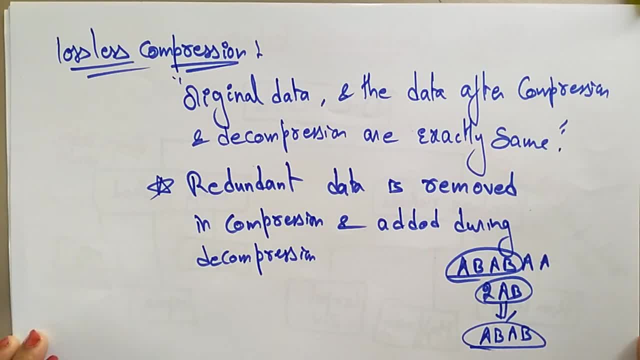 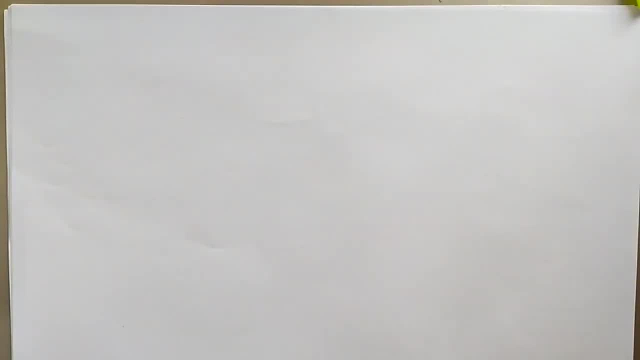 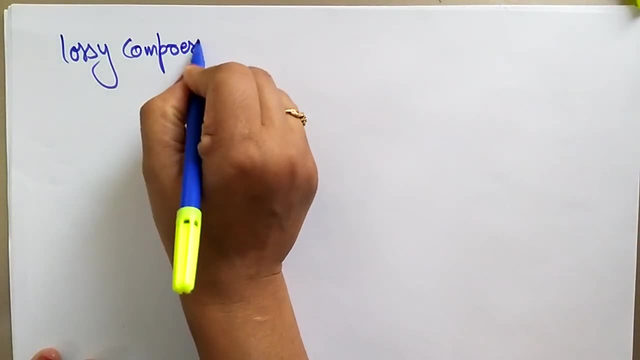 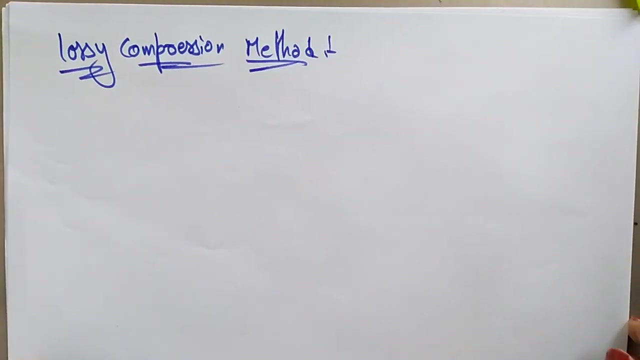 okay, so this is about the lossless compression. let me explain you about. about the lossy compression. okay, so let me explain you with the lo. what is this lousy compression? so i said lossy compression means there is a chance of uh, removing the redundant data. 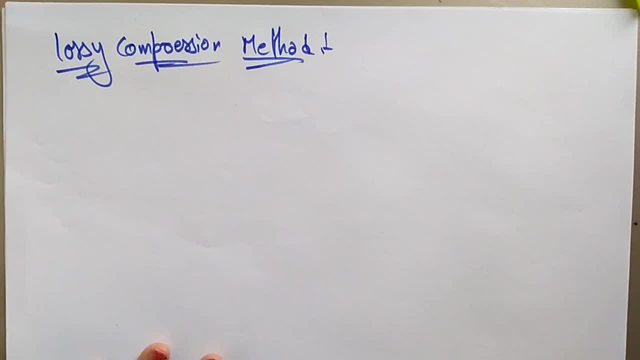 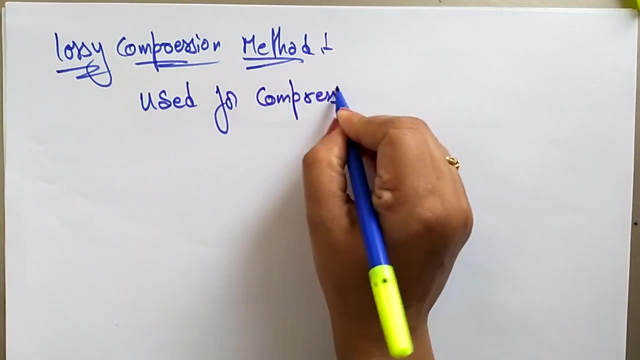 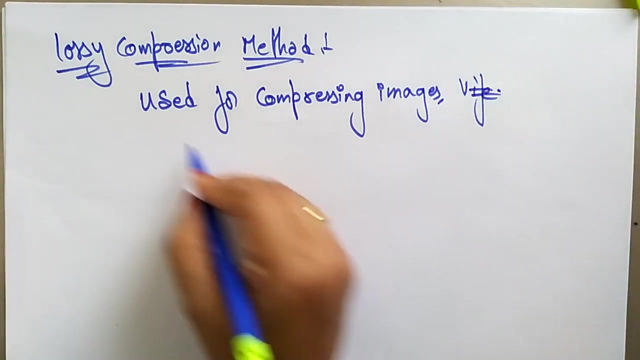 before and after the compression also okay. it is used for compressing images. used for compressing images and video files, audio files, video files, audio files: for all that, we will use a lossy compressions. so here our eyes cannot distinguish subtle changes, so lossy data is acceptable. okay, so in this cases, in the images and video files, lossy data is acceptable.